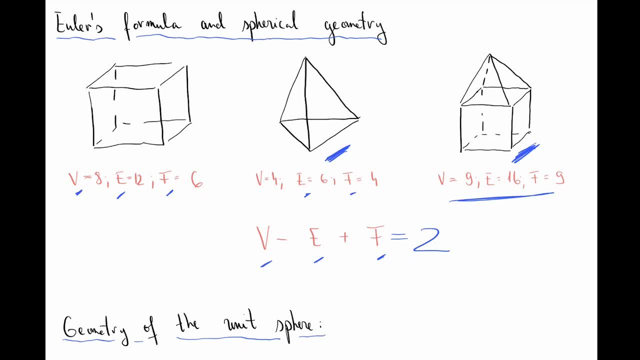 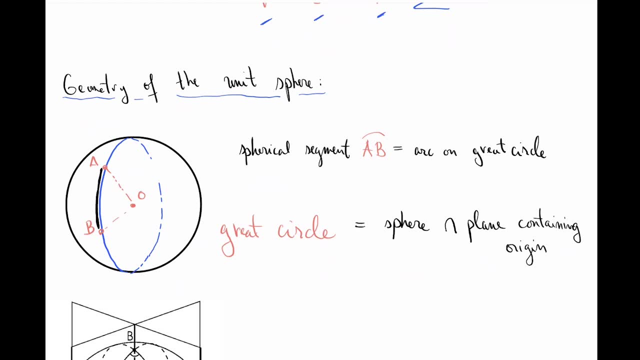 sphere. the formulas are the same, It's just that you have to rescale by the length of your radius. All right, So let us take a unit sphere and let us take two points on it, right? So in this case, a point B and a point A. And really the question is, if I can only travel along the sphere, what will I do? Well, let's take a point B and a point A. And really the question is: if I can only travel along the sphere, what will I do? Well, let's take a point A and a point B, And really the question is: if I can only travel along the sphere. what will I do? Well, let's take a point B and a point A And really the question is: what did I do? Well, let's take a point B and a point A And really the question is: what did? 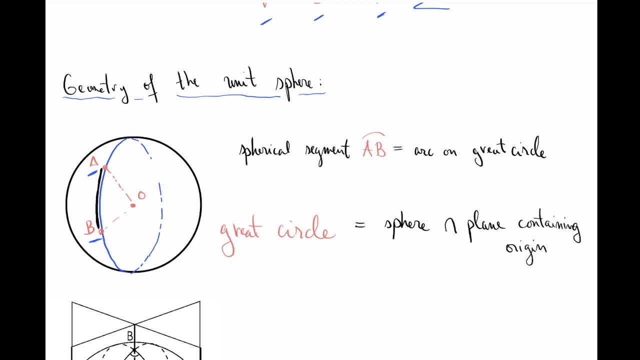 I not do. Well, let's take a point B and a point B, And really the question is: what did the two successive points create? All right, so we have this graph, and the best would be moving this curve then, And then we pick up C machines. Here you have both eight points. 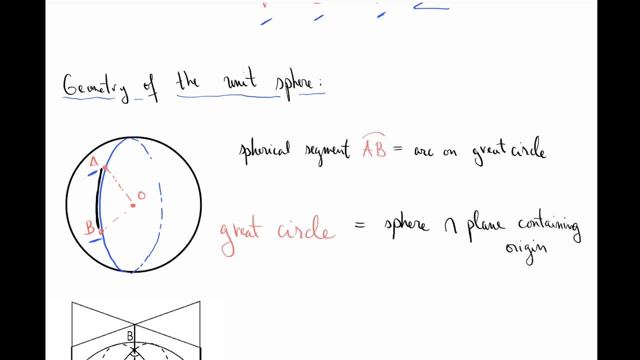 A and four points A. So the graph. infants is counting. the contribution of one of the points A and B, Theила свет councils that… to gain engagement by these two different new points, they have a nice ball last m本 sht. oops, don't get me wrong. So the graph. 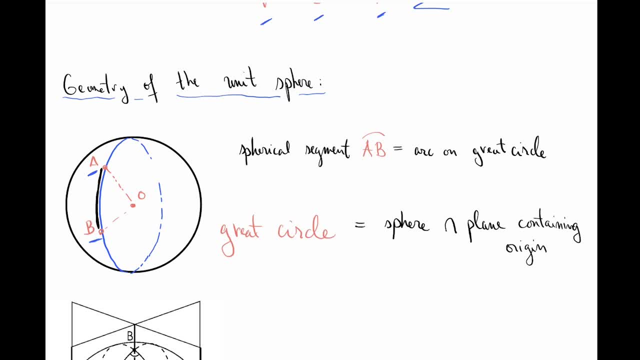 length curve is nothing but the great circle that collects the two points a and b. so how do you construct a great circle on a sphere, right? so you take the two points that you want to collect, in this case a and b, and throw in also the center of the sphere, o right, so three points form a plane. 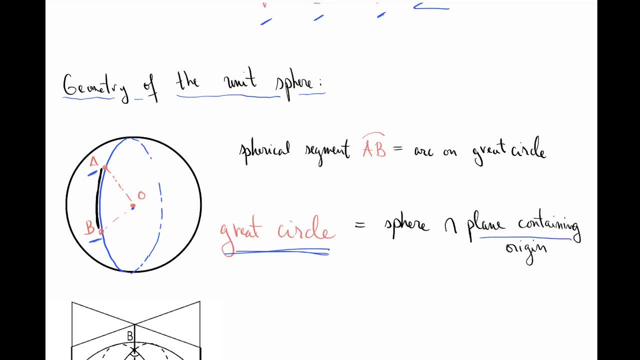 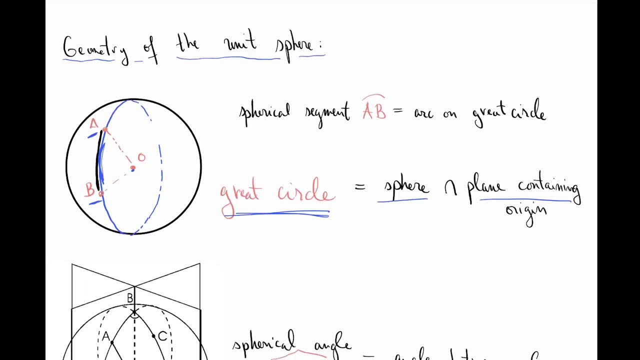 and then the intersection of the plane and the sphere is a great circle right, and then you take the arc on this great circle that joins a and b, so that will give you the spherical segment a- b or you could call it the spherical arc. okay, so that's how you construct segments on the unit. 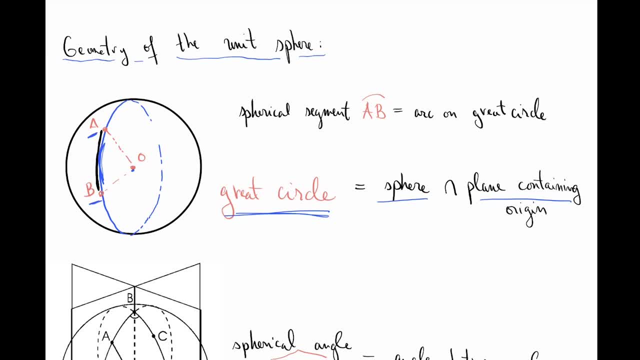 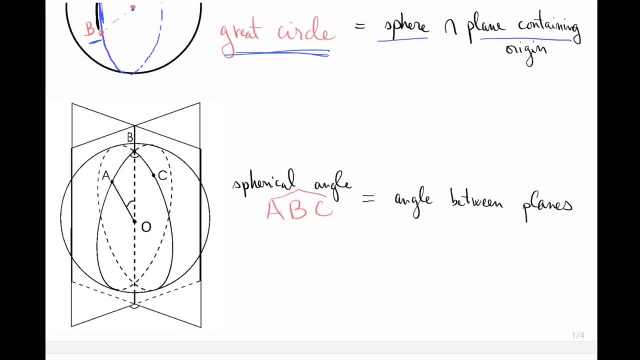 sphere right, by taking great circles. now, the other thing that you want to understand is how are angles understood in a surface, on a, on a sphere? so what's a spherical angle? right? so i take three points- a, b and c on my sphere, and the question is: how do i measure the spherical angle a, b, c? well, it's real simple. 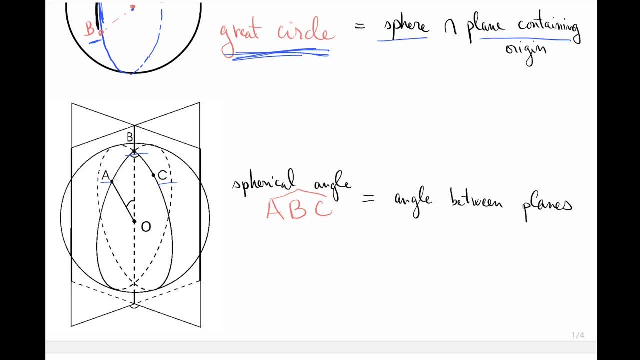 right. so here you already know that in order to understand the arcs a, b and b c right, you need to take planes that contain these points and the origin, right. so this plane here cuts out the arc a, b and this plane here cuts arc, cuts out the arc b c. right now, if i want to understand the spherical angle a, b, c 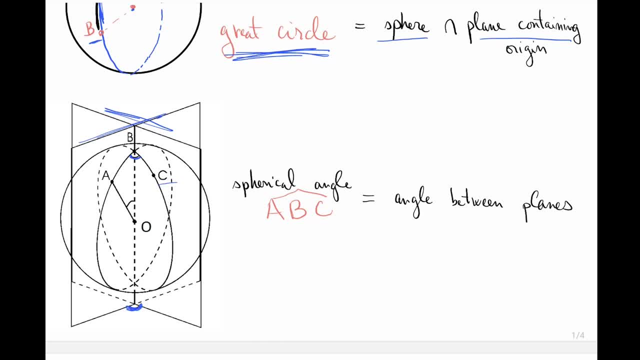 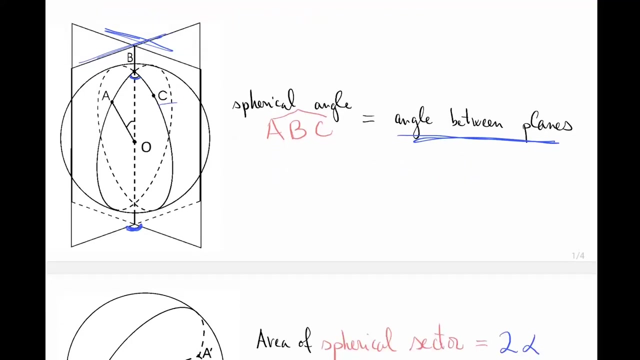 that's nothing but the angle between these two planes that i just constructed, right, so spherical angles are really angles between the planes that cut out the great circles in question. okay, good, so we understand what spherical segments are and we understand what spherical angles are. so now let's discuss areas. 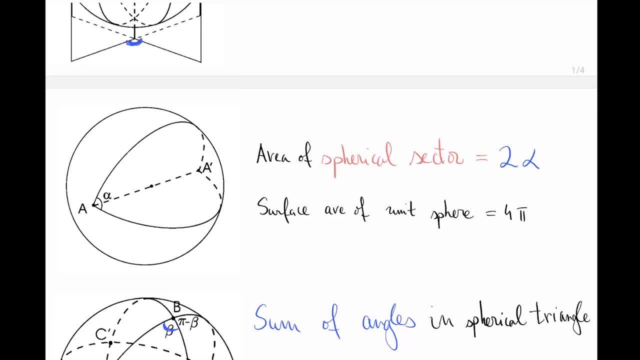 so the the most basic area, the most basic object on a sphere, on the surface of a sphere, is a spherical sector. right? so the spherical sector is the area that's cut out between two great circles, right? so you take great circles and they're always going to intersect each other and they're always going to determine a spherical 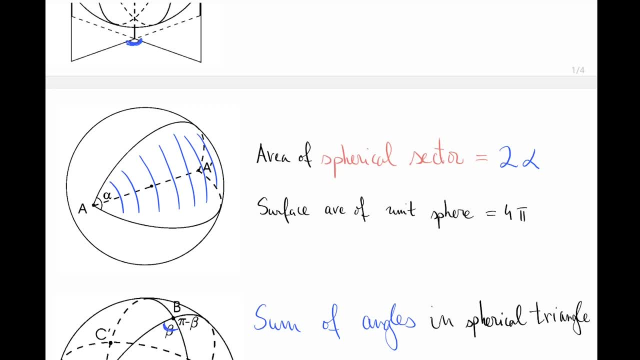 sector, right? so the question is: what is the surface area of this spherical sector? so what you immediately realize is that, whatever the area is right, of this blue shape that i indicated here, right, it's going to be proportional to the angle of the spherical sector. so in this case it's alpha. 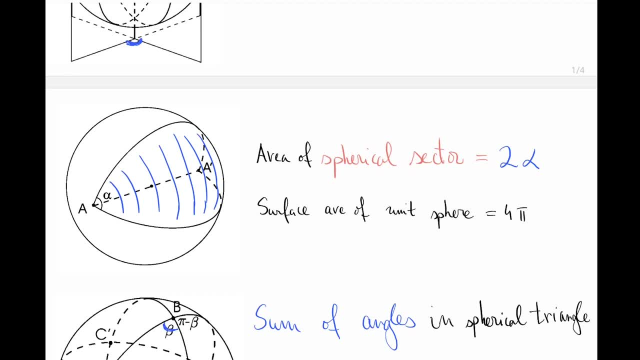 right? so now? now think about this: if this spherical sector would contain the whole sphere, then this angle would be exactly equal to 2 pi, right? so if alpha is equal to 2 pi, then the spherical sector is the whole sphere. but what's the surface area of the unit sphere? well, it's equal to 4 pi, right? so if the 2 pi angle gives 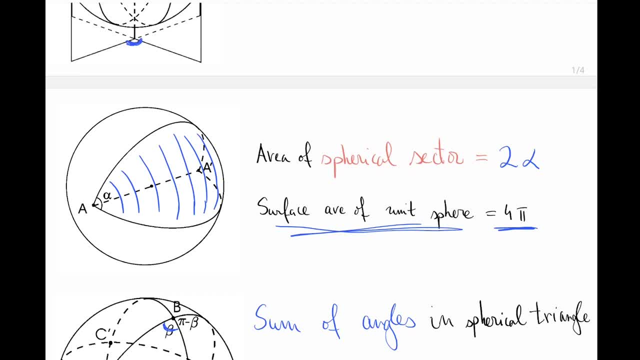 you a 4 pi surface area. if the surface area is proportional to the angle, then the area of the spherical sector of angle alpha has to be two times alpha right and also, as i said, right. so if alpha is equal to 2 pi, then you recover the full surface area of the unit sphere. okay, so now you. 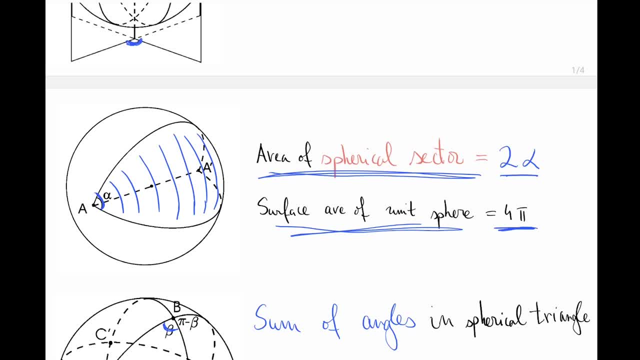 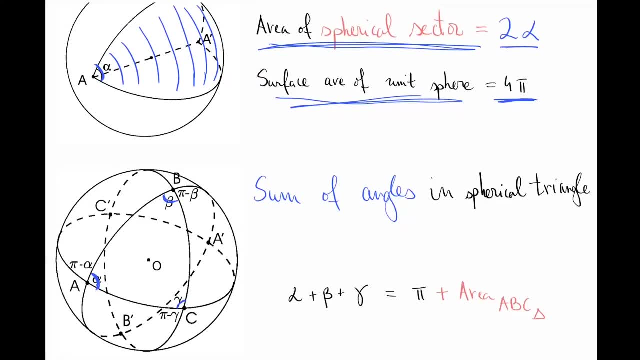 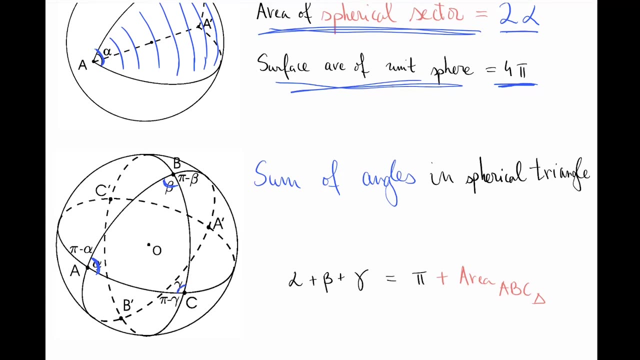 know what the spherical sector is and how you compute its area, okay. so now let me teach you something really cool about a spherical geometry that's totally different from plane geometry, okay, so take three points- in this case a, b, a, b and c- on a sphere and form a spherical triangle, right? so that means find, 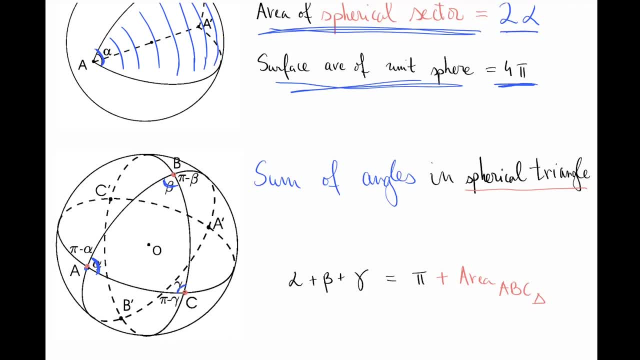 the great circles along all these three points and then join them to form a spherical triangle. so there's, uh, the most basic question that you could ask. uh is something that you do also in plane geometry- what is the sum of the angles, uh, in spherical angles in this triangle, right? so in this case, 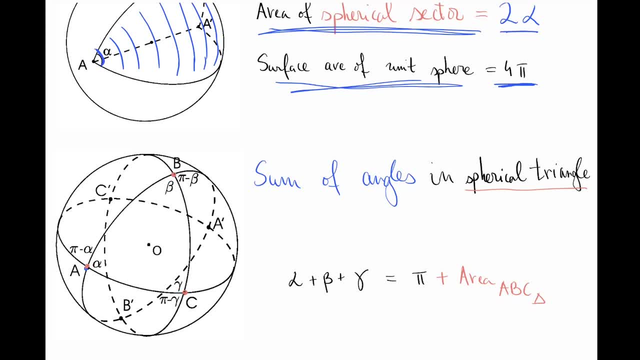 we have alpha, beta and gamma, the three spherical angles. so you ask yourself: what is the sum of these angles? well, in plane geometry, the answer is always pi, right? so in spherical geometry, however- and this is the first difference, perhaps, between plane and spherical geometry- it's pi plus the area of the triangle, right so. so there's this area that the 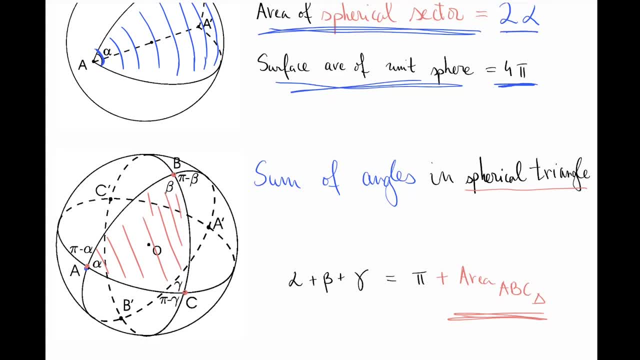 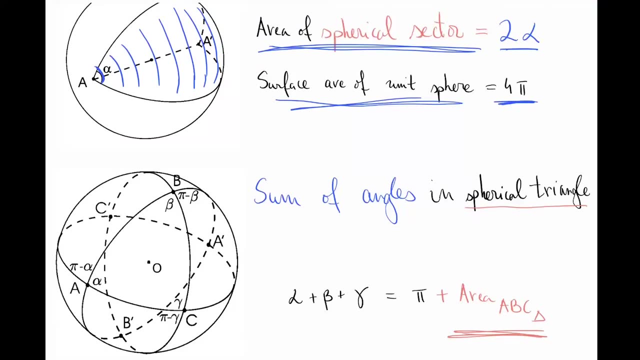 triangle covers, and then the sum of the three angles is equal to pi plus the area. so i'm going to prove you this really cool fact and all you need to understand, uh, and so the all that goes into the proof is what we just understood. so the area of spherical sectors, okay, so how do you show? 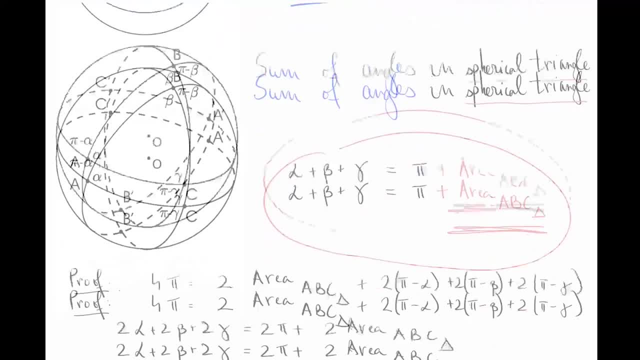 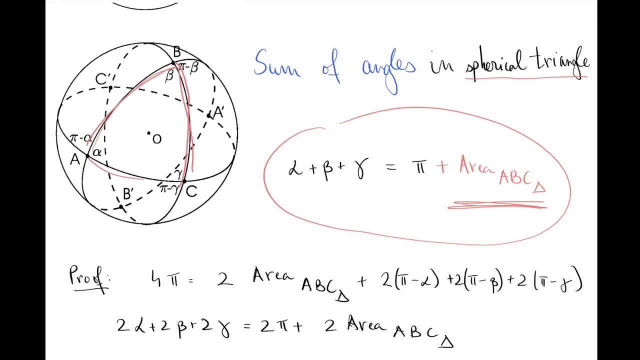 this nice formula here. well, what you need to do is is what already on the diagram: right so, extend the sides of this spherical triangle, uh, as much as you can, right. so, in other words, draw up the great circles that give you the sides, right. so if you do this, then what you will see is that on the 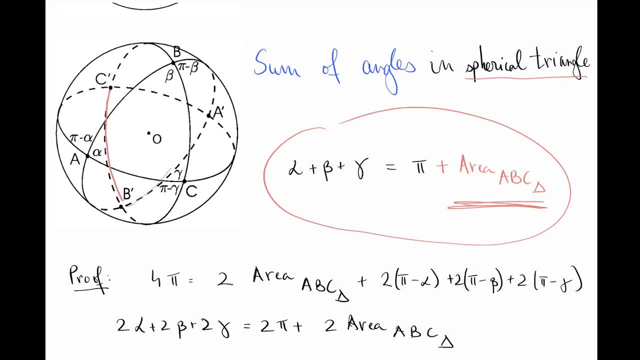 other side of the sphere, you will see this triangle- a prime, b prime, c prime- that is congruent to the original a, b, c triangle. okay, so why am i telling you this? well, because what you get is a partition of the sphere that is going to be extremely useful for us, right? so what? 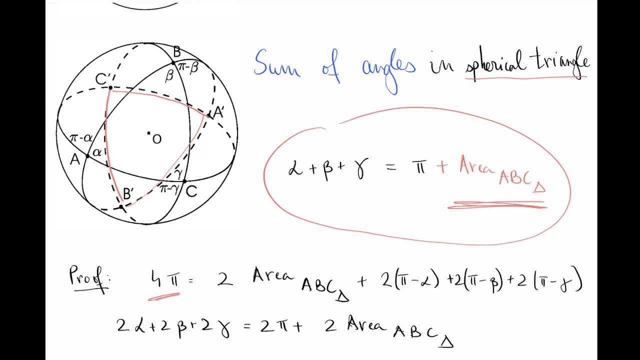 is the total area of the unit sphere? well, it's 4 pi, right so, since the radius is one and the total area is 4 pi, okay, so now these three great circles have partitioned the sphere in a really cool and useful way, right? so there are two triangles here that are congruent to each other, right so? a, b, c and a prime. 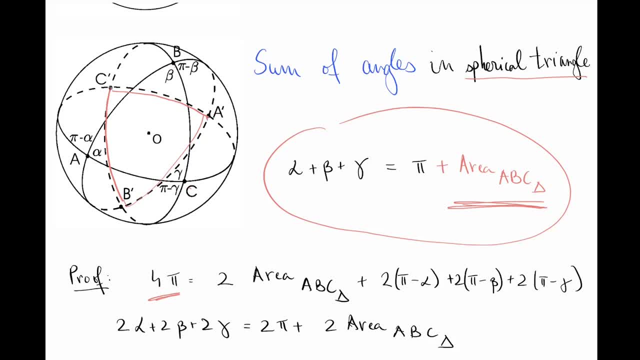 b prime and c prime right. so if i want to partition the area, i count twice the area of a, b, c, right, so that accounts for the triangle here in the front and the triangle in the back. now, in addition- and it takes a minute for you to see this, but it's not too difficult- the total area that is left. 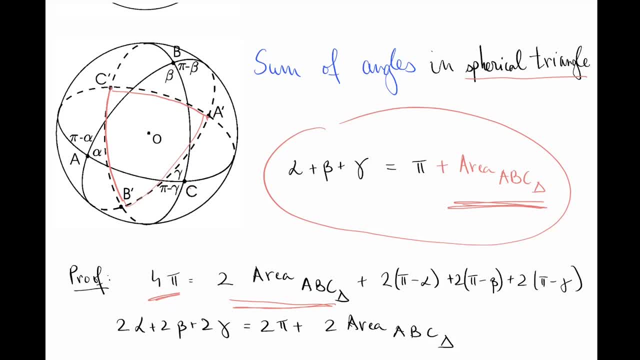 comprises of the area of three spherical sectors. right, so the first spherical sector is the sector you get from this outside angle to alpha. right, so it starts over here, and when you peel it off, you get this spherical sector here. right, so next the next one. i won't draw it in because it will. 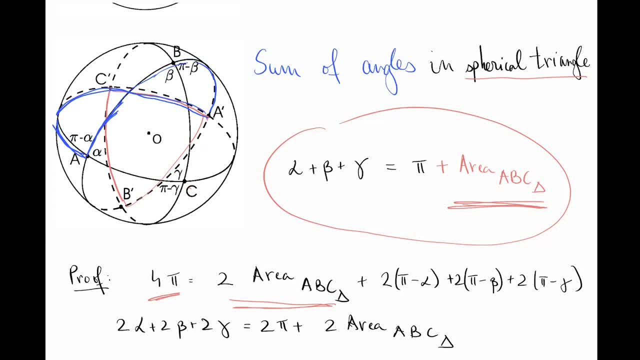 be difficult to see, given everything that's already up here. so the next part that we haven't accounted for starts with this corner right. so this angle: pi minus gamma. when you peel off this sector right, you will see that you only have one more uh sector left, and that is the one that starts with. i mean, it starts from this, this: 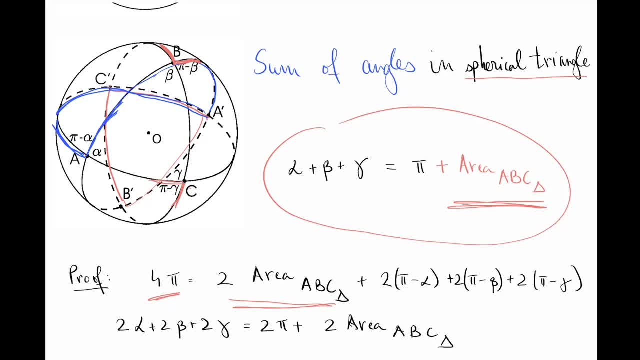 corner up here right, and it has angle pi minus beta. so these are all spherical sectors and their areas account for two pi minus alpha, two pi minus beta and two pi minus beta and two pi minus gamma right. so all in all we get that four pi. the total area of the sphere is 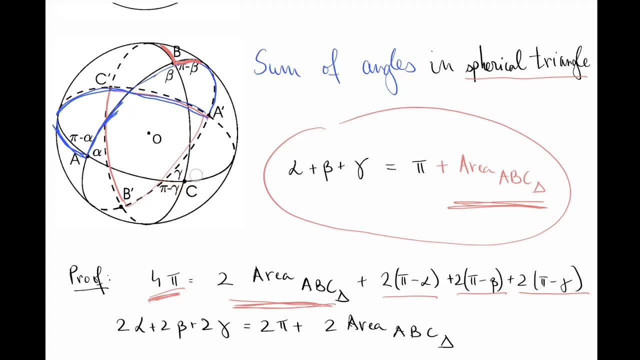 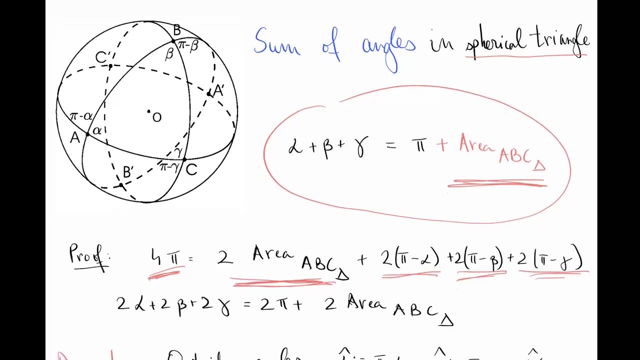 equal to twice the area of our triangle abc. so let me erase everything here so we go back to the beginning, right? so twice the area of abc plus one of the areas of the spherical sector, the other area of spherical sector and the third one, right? so if you add everything up, you get 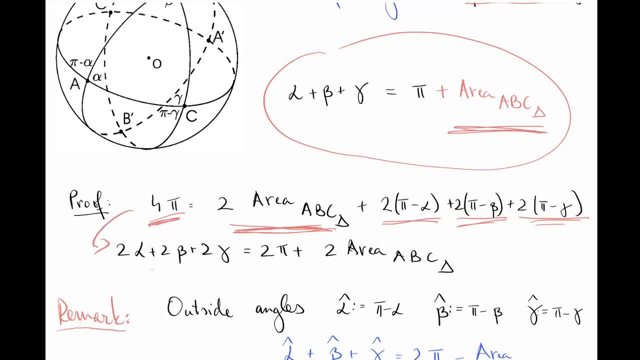 do a bit of algebra, right. so from here to here, you get two alpha plus two beta plus two gamma is equal to two pi plus twice the area of abc. you divide by two and then you get the formula that i have over here, right? so the sum of the 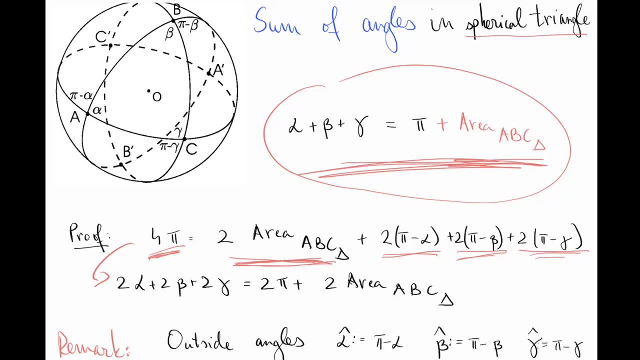 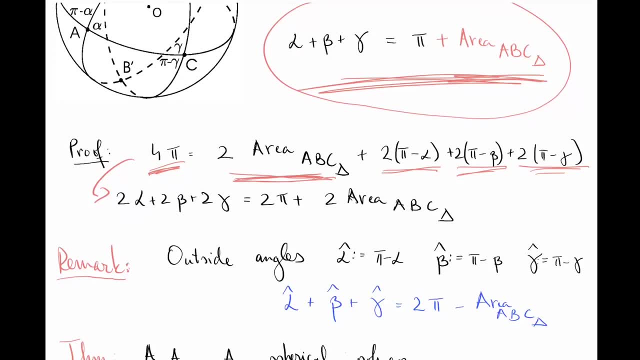 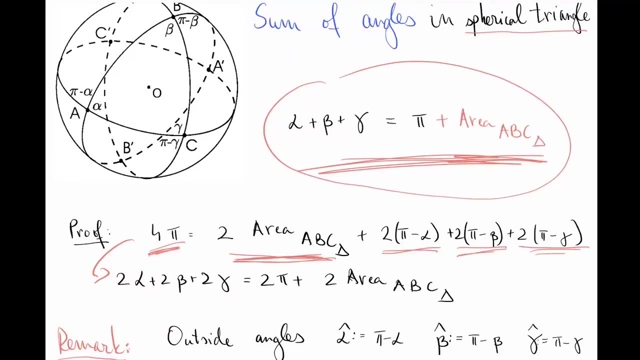 angles in a spherical triangle is pi plus the area of the triangle itself. okay, so something that will be really useful for us in the proof of euler's theorem is also looking at the outside angles, right? so what are the outside angles in a spherical triangle? it's the same as in the plane, right? so in case of this triangle, abc, the outside angles are this one: 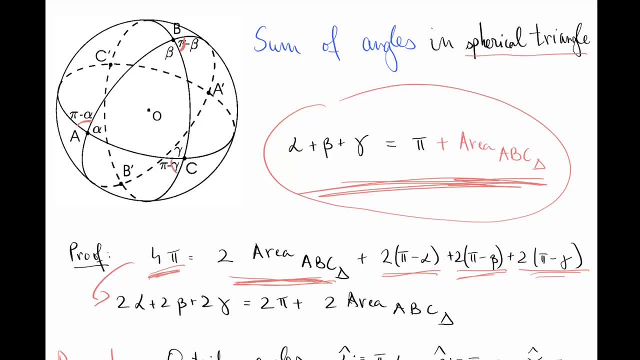 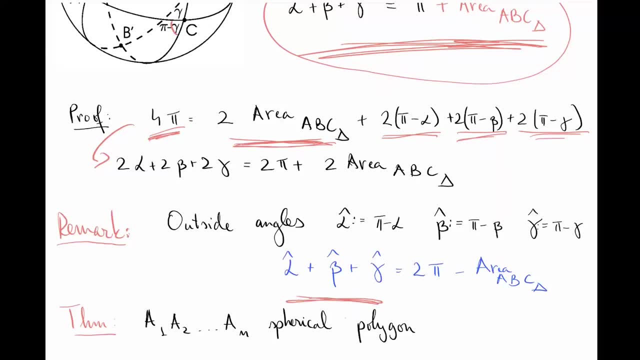 this one and this one over here, right? so the an angle plus its outside angle always add up to pi. so if you want to get the sum of the outside angle, so in this case alpha hat, beta hat and gamma hat, if you sum them all up, it has to give you two pi minus the area of the abc. you get this a. 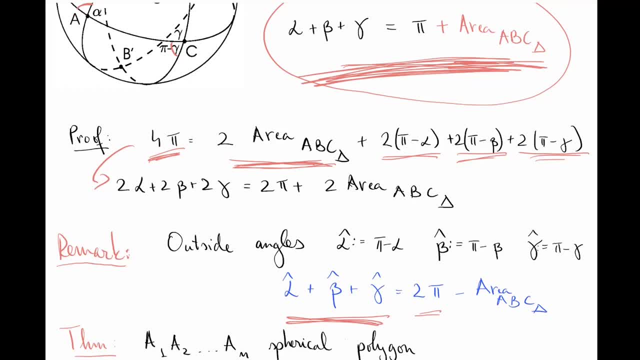 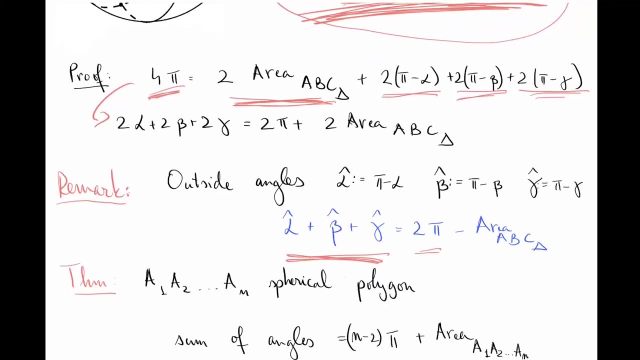 very quick formula over here on the top. okay, so you can go really quickly from triangles to polygons, right? so what are spherical polygons? well, you take up end points on the sphere and you join them by spherical segments. and you might ask yourself again: what is the sum of? 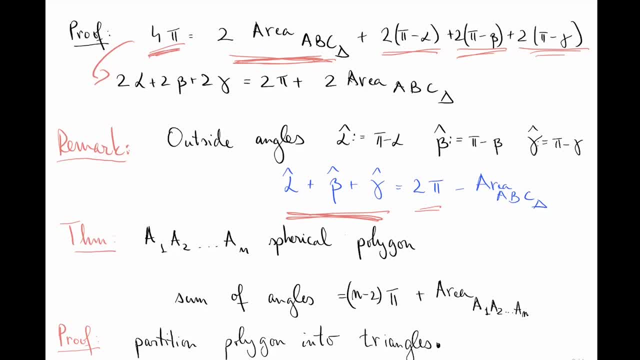 all the interior angles, or all the angles. well, it will be the same as in plane geometry n minus 2 pi, but again you have to add in the excess area, so area of the full spherical polygon, right and again. how do you prove this? you prove this the way you prove that, in in case, 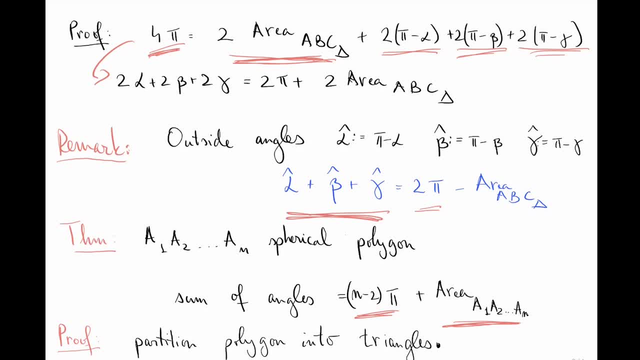 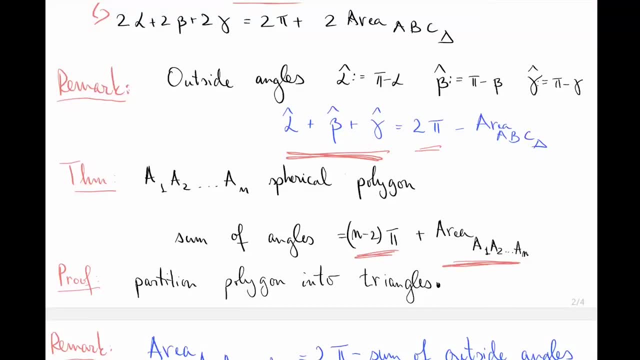 of the plane right, the sum of the angles is n minus 2 times pi. you partition the polygon into, in this case, spherical triangles and then you know the formula for each spherical triangle. you add up all the formulas in catch avis triangle and then it will give you. 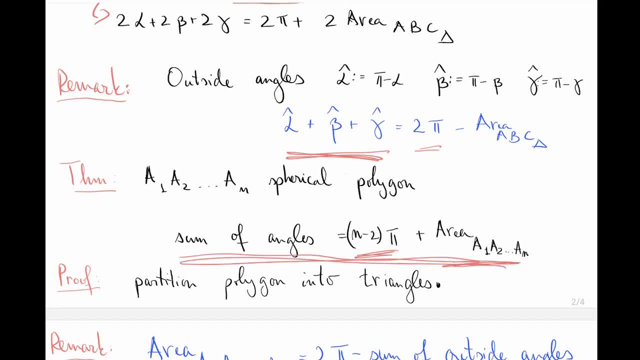 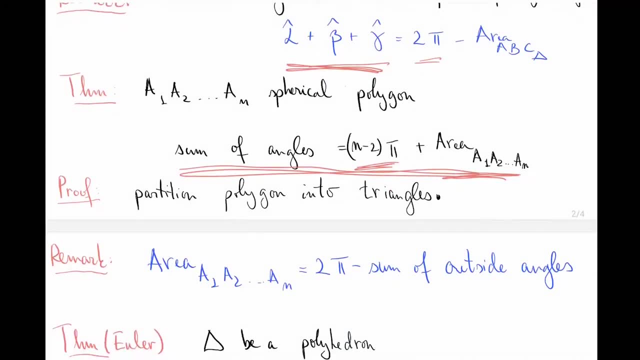 this formula here, so i'll leave the details to you. it's quite simple and again, you also get a formula for the sum of outside angles. so i will write that here in this form, so you can express the area of the spherical polygon as two pi minus the sum of all. 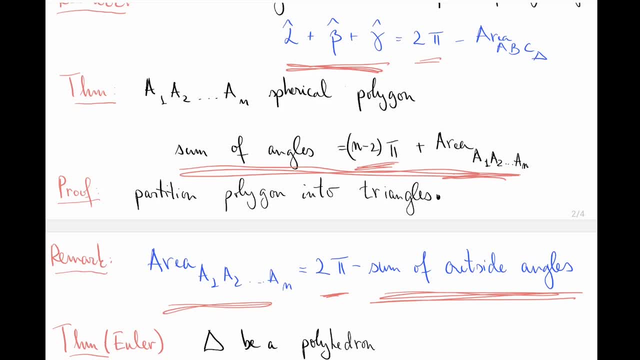 the outside angles. okay, good. so now that you understand this, you will be surprised to know that we are ready for a new table. we're going to grow into overarching and sphericalymm, entrepreneurial, ready to prove Euler's theorem right. So let delta be our polyhedron. as complicated as they. 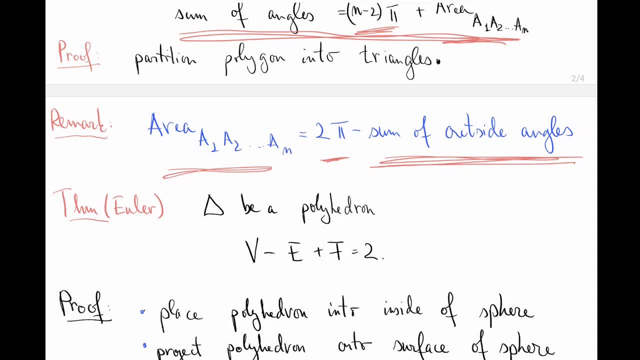 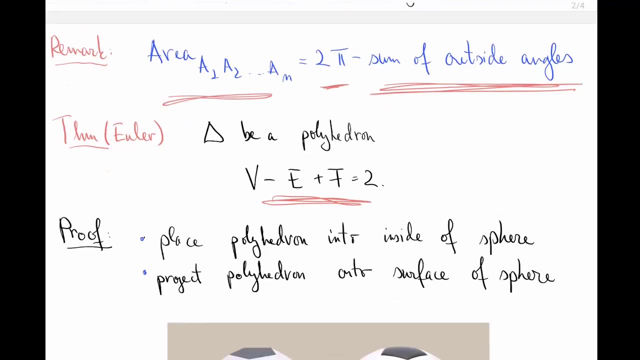 get, and then number of vertices minus number of edges plus number of faces should be equal to 2.. Okay, so how does this have anything to do with spherical geometry? Well, let me show it to you. So you take your spherical polyhedron and put it inside your sphere, right? So maybe you have to. 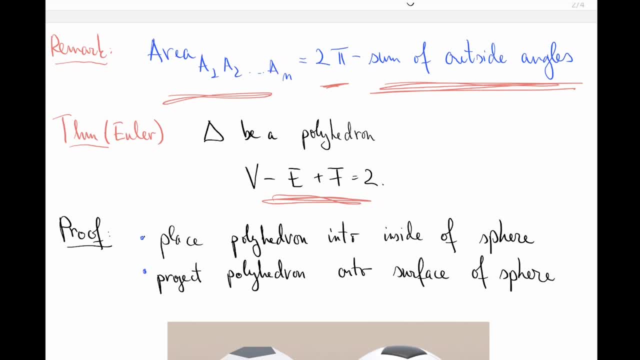 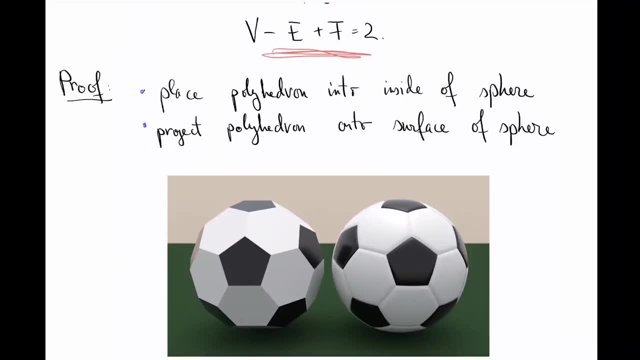 zoom it down a little bit and put it inside the sphere and once it's inside the sphere, project it onto the surface of the sphere. So this sounds quite complicated, but I guarantee you that you've seen this before As a matter of fact. right? so this is how the icosahedron becomes the soccer. 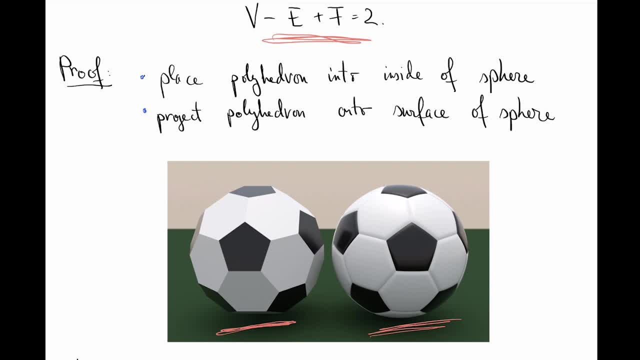 ball right. So place the icosahedron inside A sphere and project it onto the sphere, and then you get the soccer ball. Okay, so we will be working with the soccer ball right. So what? the really important thing here is that, once you do, 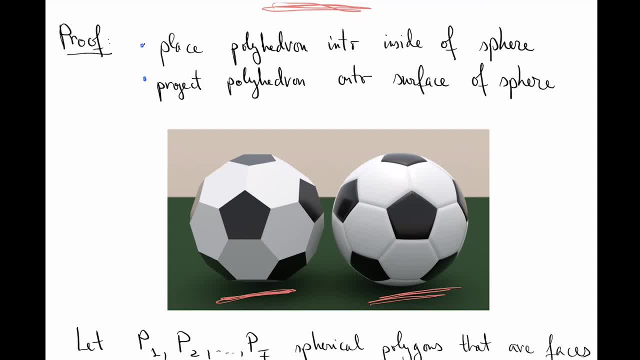 this: the polyhedron will cover the whole surface area of the unit sphere, And then you get a bunch of extra geometry that you wouldn't see unless you project it onto the sphere. So what you're going to do is you're going to project it onto the sphere and then you're going. 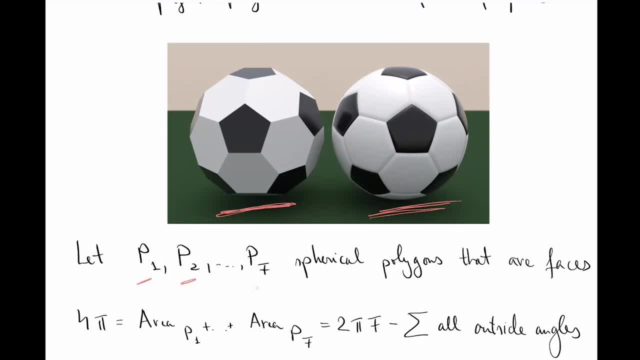 So what do I mean? So let P1, P2, and PF all the way to PF, the spherical polygons that are the faces of our spherical polyhedron. right So in case of the soccer ball, right. so P1 to PF will. 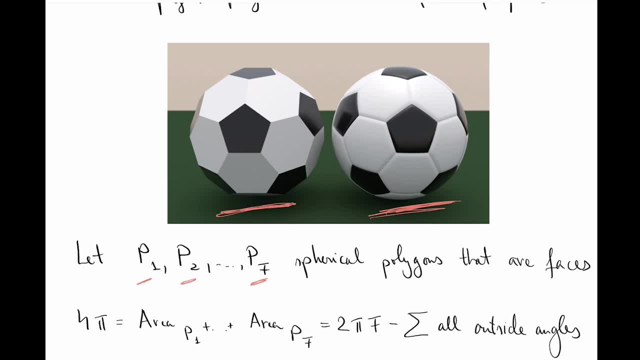 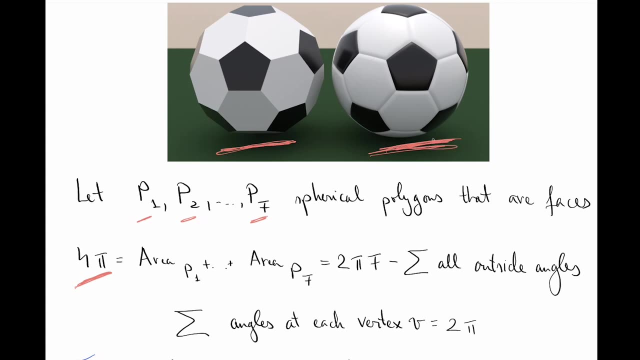 be a bunch of spherical hexagons and spherical pentagons, right? So the total area of the unit sphere is equal to 4.. I can express that using the partition. In case of the icosahedron, right, it will be the partition. 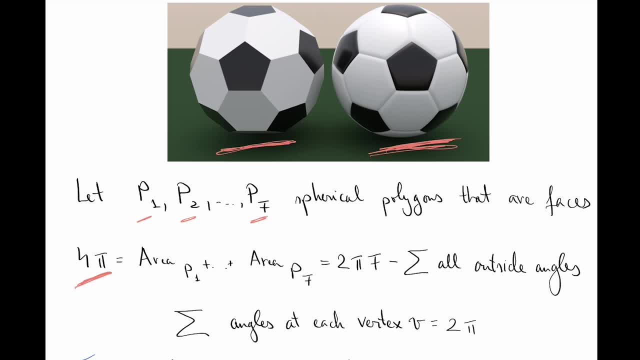 that the soccer ball does to the sphere, right? So it will be the area of this bunch of, in case of the picture, right? So I have a bunch of areas of hexagons and a bunch of areas of pentagons. 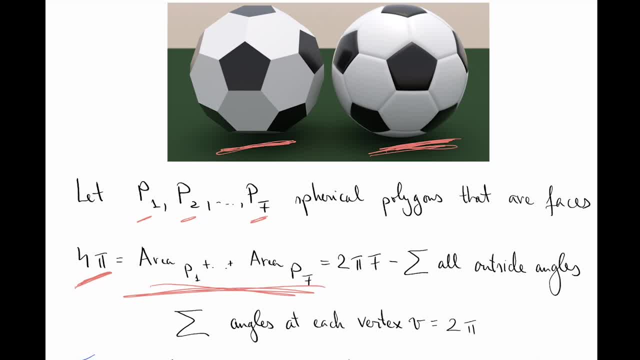 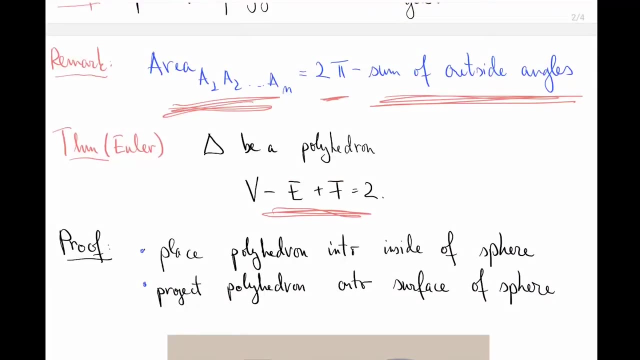 right, So I do that over here. Okay, so now I use the formula that I just learned in terms of outside angle, right? So each polygon, the area you can write up, so let me just roll back real quick- the area of that polygon you can write up as 2 pi's minus the sum of outside angles for 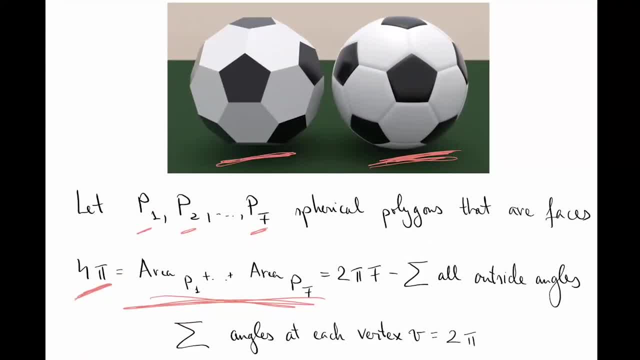 that polygon right. So in case of this spherical polyhedron, we sum up all the areas of the polygon so that will be equal to 2 pi times the number of faces minus the sum of all possible outside angles that can appear right. So this outside angle, this outside angle. 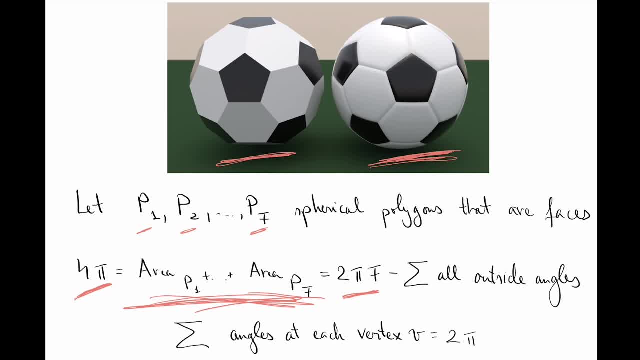 sorry, that's not an outside angle. so this outside angle, this outside angle, this outside, all possible outside angles that you can write down. Yeah, those are not outside angles either, right? So things like this, right? So in case, 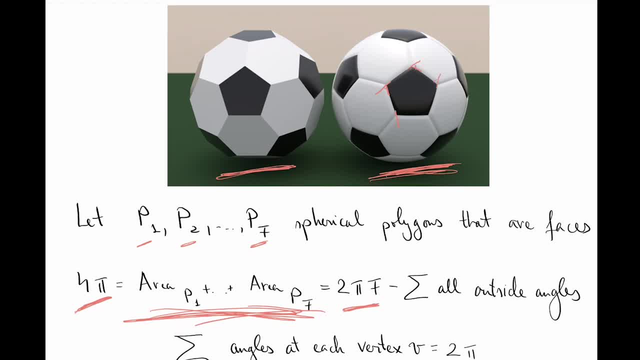 of this pentagon over here, all right? So maybe I can write down all the outside angles for just for this pentagon, right? So this is just one pentagon here. Do it for all the hexagons, pentagons. 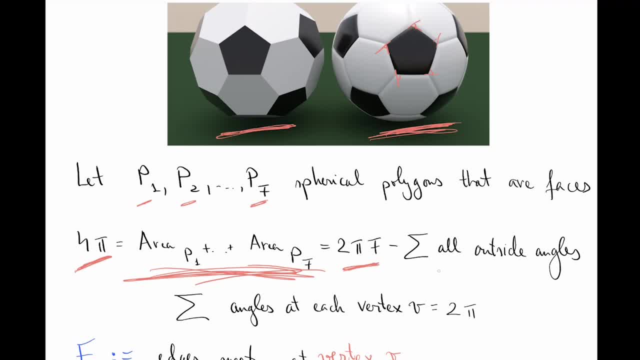 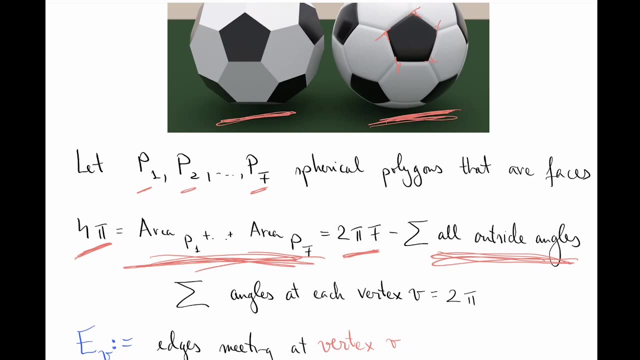 and then all those measurements for all those angles will go in this sum here. Okay, good, Okay. so let's look at this sum here a little bit differently. Okay, so what happens if I sum up all the angles of my polyhedron at each vertex, v right? 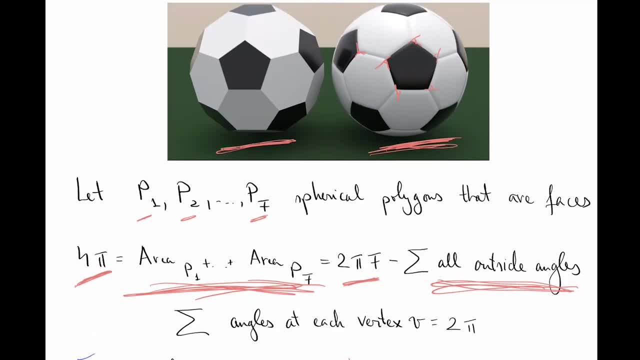 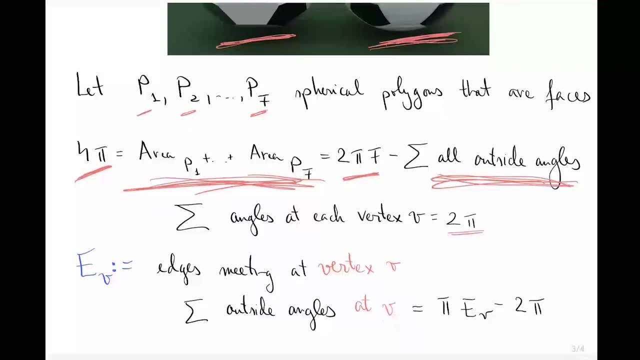 So if I just focus on a vertex v and I sum up all the angles, not the outside angles, the angles right, So this will sum up to always to two pi, okay, Okay, so let me denote by e v the number of edges meeting at a specific vertex v right. 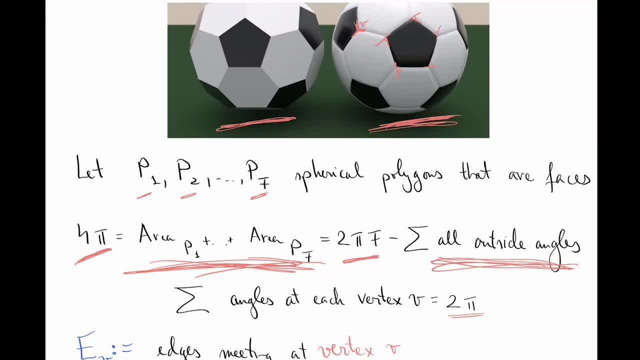 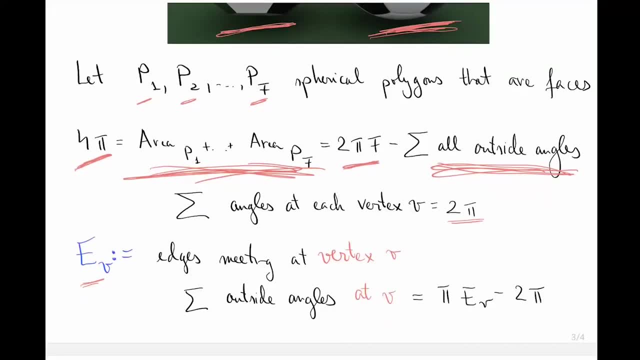 So if I call this v, let e v the number of edges meeting at v, right. So in this case it's one, two, three. Okay, so since the sum of the angles meeting at each vertex is two, pi, you know a very basic algebra operation. 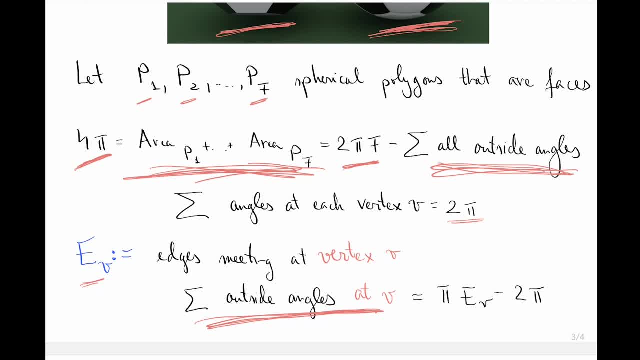 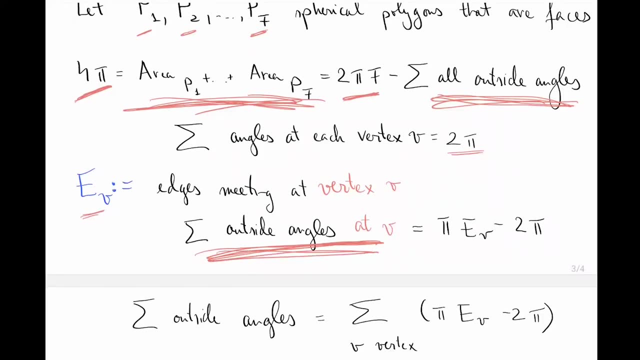 tells you that the sum of the outside angles at v is equal to what? Well, it's equal to pi e v minus two pi. Okay, good, So now what do I do? Well, I sum up the sums along all the vertices that I have right. 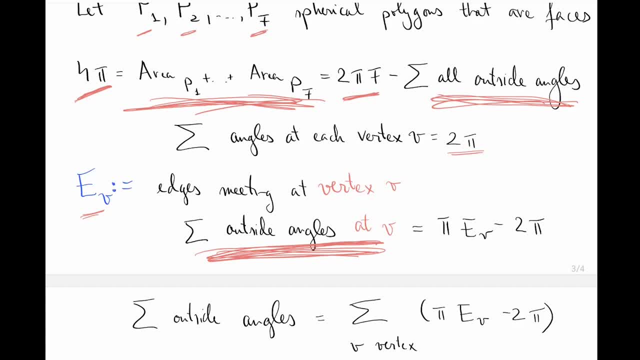 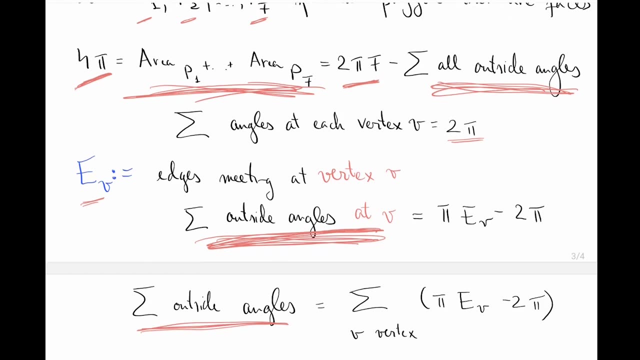 So you have all the outside angles at v, and now you summing up across v, v being a vertex in your polyhedron right. So what will that give you? Well, it will give you all possible outside angles. Okay, good, and the right hand side. what you get? 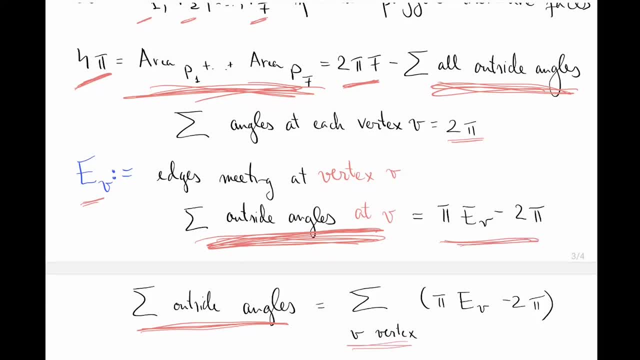 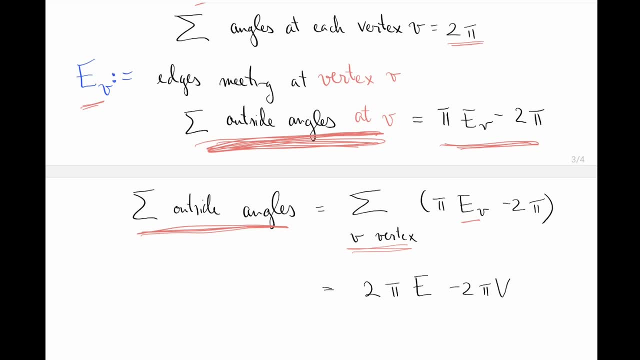 Well, you get these expressions summed up, right. So you get these expressions summed up across all vertices, Okay. so what's going on? So e, v is the number of edges meeting at a fixed vertex, v. Okay, but every edge has two ends, right?